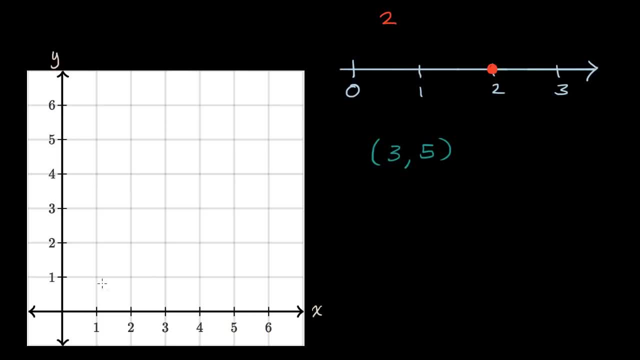 How does that, or how can these two numbers, be represented as a point on the plane, Or how can these tell you where a point on the plane is? So let's first get a little bit of terminology out of the way. So what we have here, this is often known. 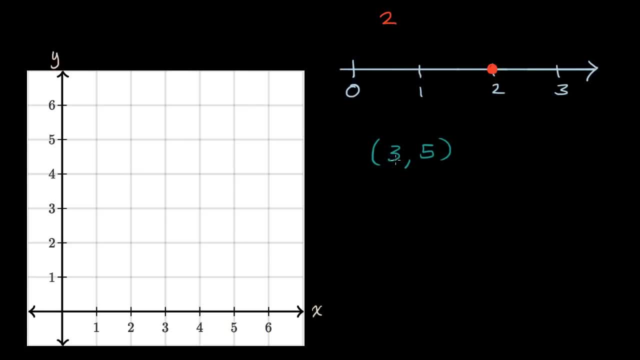 as our coordinate plane, These two numbers you could view as our coordinates. Let me write this down. These are coordinates. These black lines are known as the axes. Each one is an axis And the one that goes left right here this is known as the x-axis. 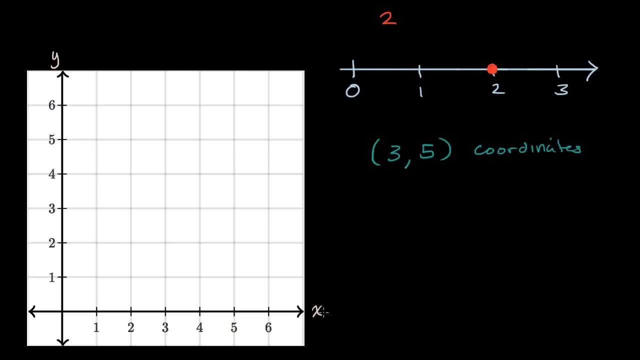 or it's typically known as the x-axis. In the future it might be called other things And the one that goes up down in the vertical direction. this is typically known as the y-axis. As you go further in math, we might call it other things. 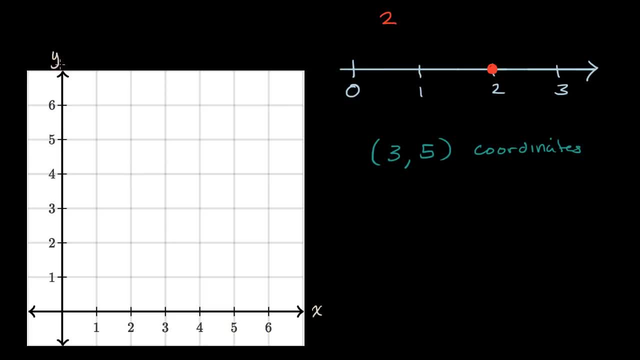 but most of the time it's going to be called the y-axis. So how does three comma five, how do these coordinates specify a point on this plane? Well, the way that we typically work it through, the standard way that people will interpret these points. 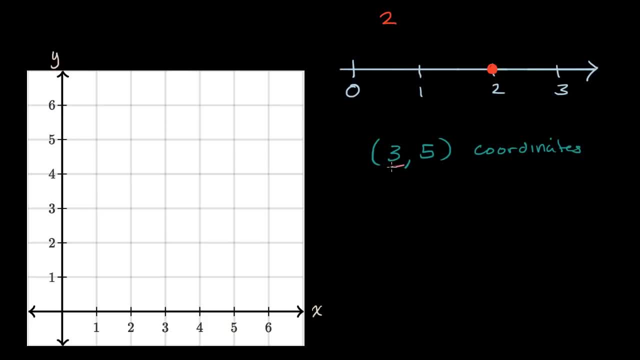 is they'll say: all right, this first coordinate, this is our x-coordinate, This is our x-coordinate. You can view it as: how far do we move to the right along the x-axis? All right, so what you would do is you'd say: 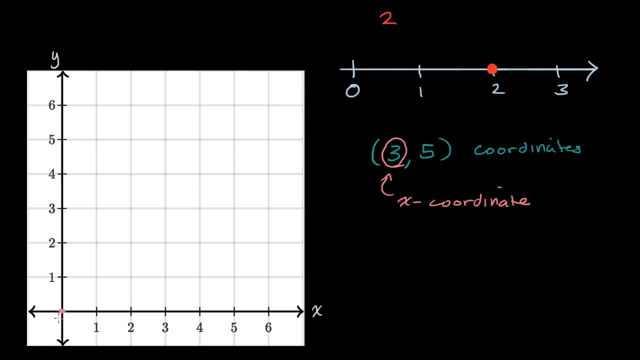 all right, I'm going to start right here, where my axes intersect, And I'm going to go three to the right: one, two, three. So my x-coordinate says: all right, my point is going to be- is going to be- this far to the right. 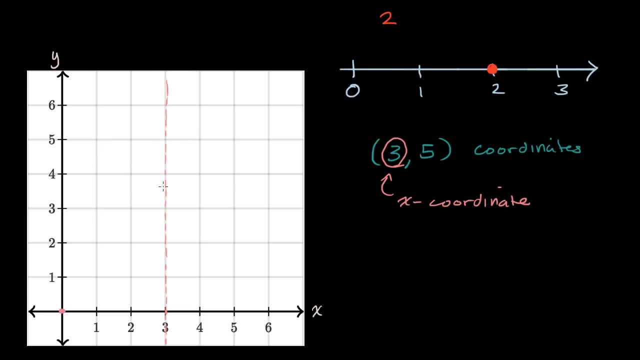 This far to the right. So it's going to be somewhere on this vertical line, this dotted line that I'm showing. Everything on this vertical line has an x-coordinate of three. Now what's the y-coordinate? or another way I should say it. 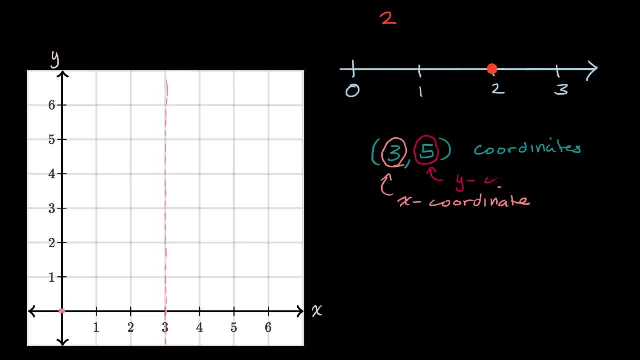 the second number right over here. this is the y-coordinate. Y-coordinate- This tells us how far do we move up. So one way to think about it: you could start back at where the axes intersect. This point is actually called the origin. 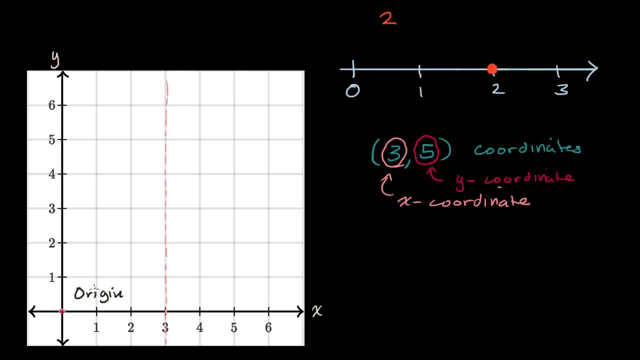 Let me write that down. That is the origin. And so, starting at the origin, move five up: One, two, three, four, five. So everything on this horizontal line that I'm drawing has a y-coordinate of five. So what point uniquely has both an x-coordinate of three? 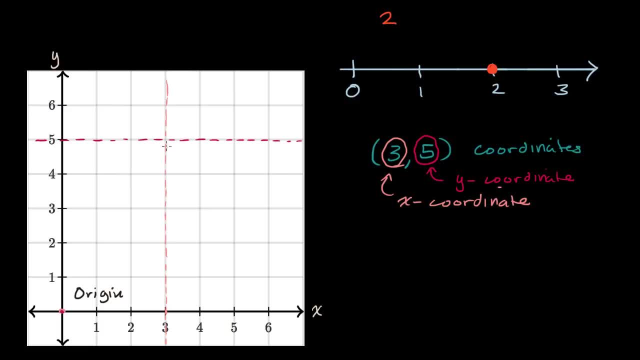 and a y-coordinate of five. Well, you could see where those two lines intersect right over here. Actually, let me do that same blue color that I wrote the coordinates in. So this point right over here, it has an x-coordinate of three. 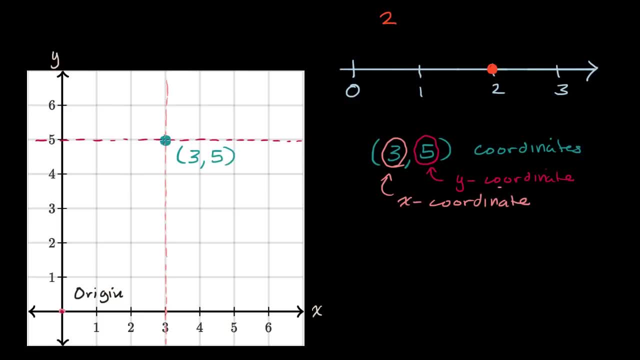 and it has a y-coordinate. It has a y-coordinate of five. That is the point three comma five. Now, what is the coordinates of the origin? Well, the origin is zero to the right of the origin and it's also zero above the origin. 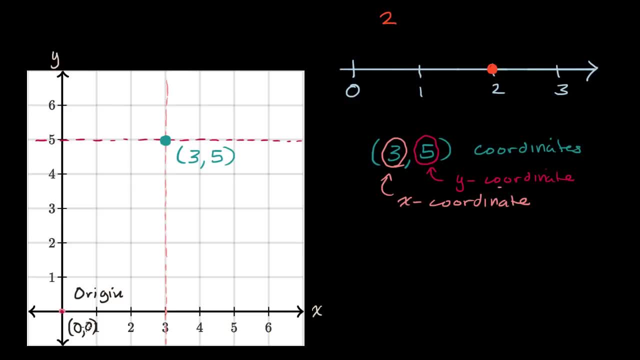 So the coordinates there, the x-coordinate is zero, The y-coordinate is also zero. Let's do a few more examples. So let's say that I wanted to plot the point two comma five. Why don't you pause this? Let me use a different number. 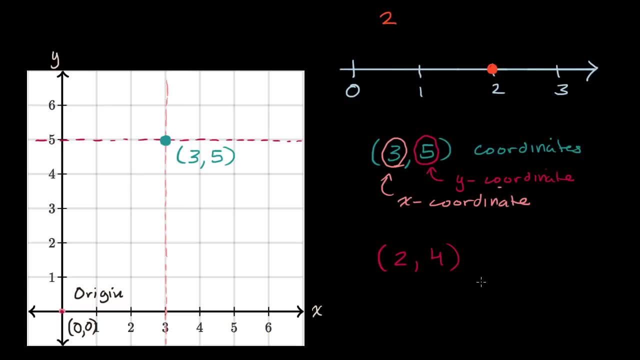 One comma four. Why don't you pause this video and think about where that point would be on this coordinate plane? All right, let's do it together. So the first number is going to be our x-coordinate. It tells us how far do we move to the right. 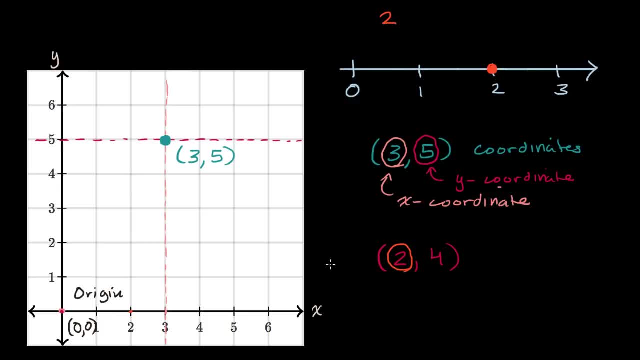 So we move two to the right And then our second number says how far do we move up. So first we're gonna move two to the right And then we are going to move four up. So you could say one, two to the right. 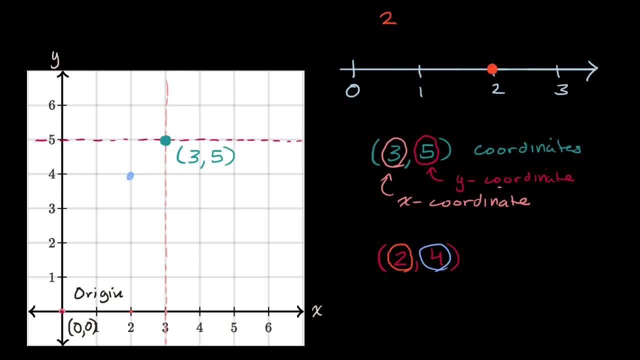 and then one, two, three, four Right over there. This right over here is the point two, comma four. Notice it's x-coordinate how far to the right of the origin it is. that is two, And it's y-coordinate how far above the origin is. 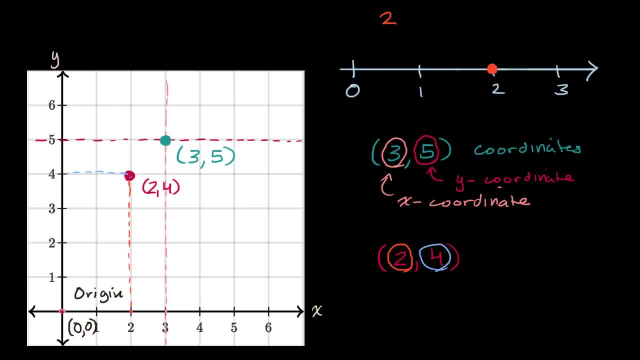 that is four. Now let's go the other way around. Let's say that I were to give you, if I were to give you, this point right over here, what would its coordinates be? Pause the video and try to figure that out.